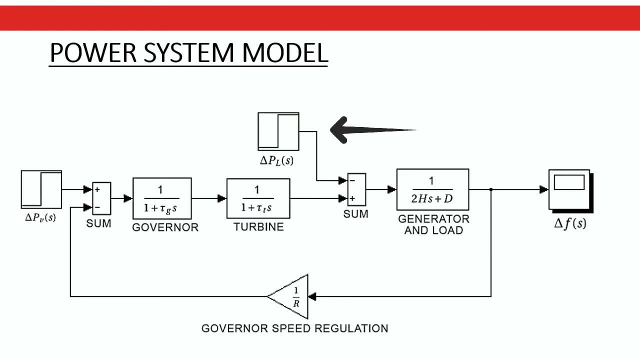 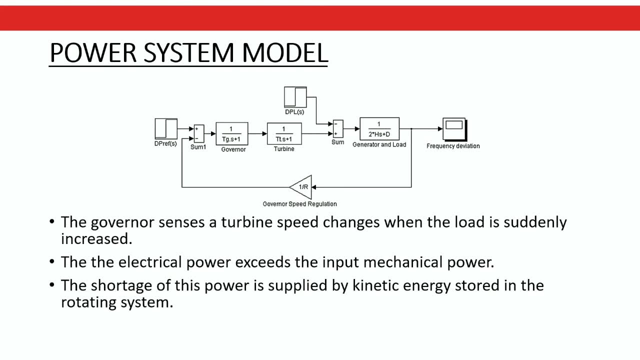 generator and load. This is the reference input and this is the load change that we are going to consider, And this is a feedback system. So the governor is a system that detects the speed of turbine and that, and in case, if the and it supplies the energy that is required for the turbine. So what we are going to do is we are going to design a state space equation for the, for the systems. 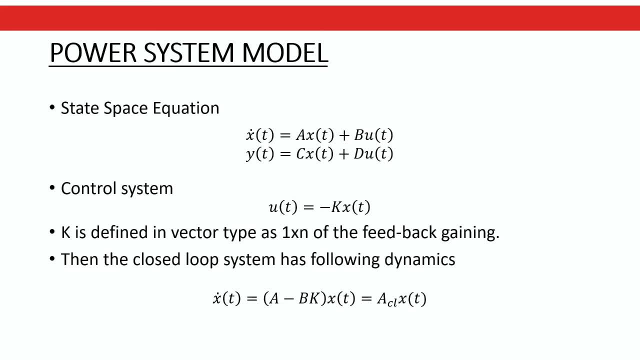 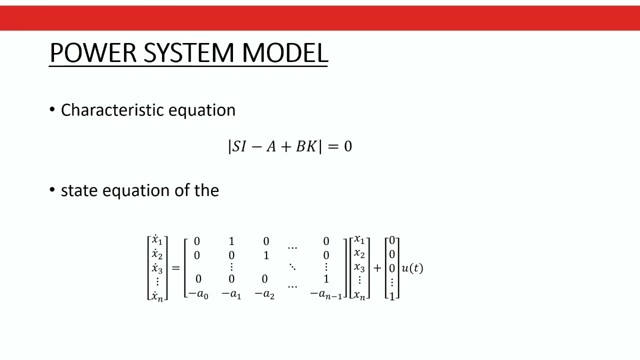 For that system. So the state space equation is the standard state space equation is this one: And if we are considering a feedback system that is u of t equal to minus k of x of t, So we just substitute this in the x dot of t equation and we get this equation, And this a minus b k is known as a closed loop. With this, the. with this, the characteristic equation is si minus a plus b k equal to zero. So if we solve this characteristic equation, we get a closed loop. 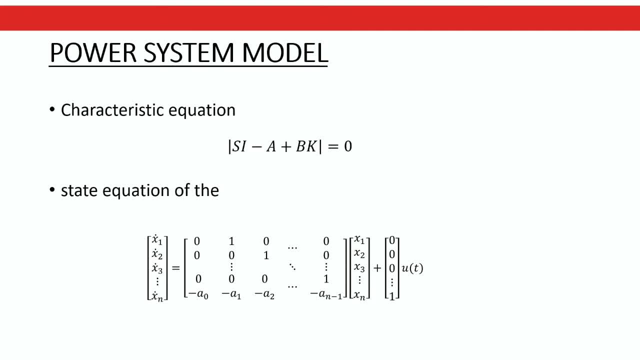 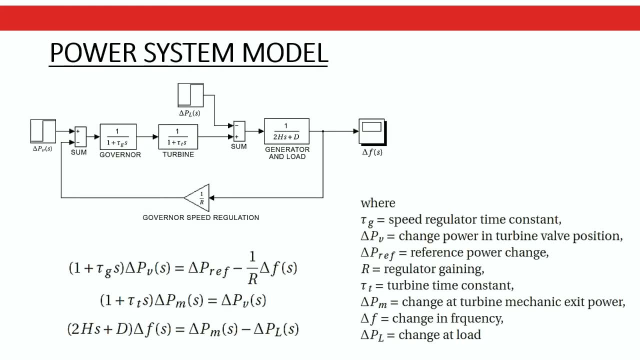 And we can arrange that in a standard state space matrix equation form And this is a standard form. So right now we are going to set up our set of equations in this form. So the control, mainly the governor and turbine and generator and load and the feedback, the transfer function of these elements are already defined and we are not going to this. So the equations, if we are considering the output of governor as delta pv, output of turbine is delta pm and output of generator is delta pm. 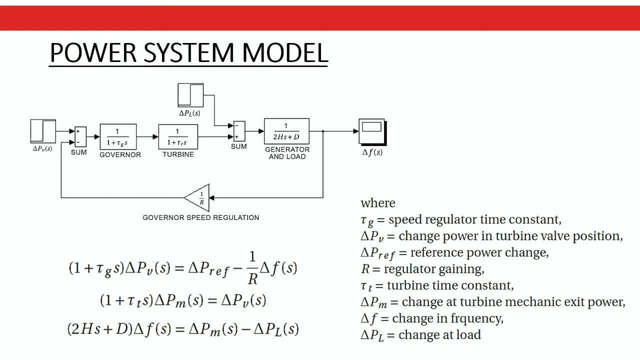 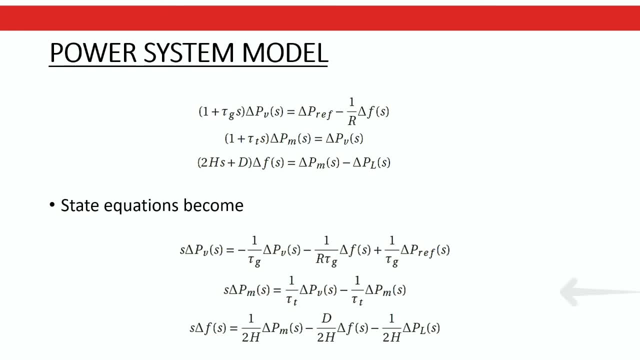 and load as delta fs. this delta fs is required, is needed for the feedback also. so, uh, this equations. after rearranging we get this and these equations are in this s domain. now we are going to transfer this into the t domain. so when we convert this into t domain, the s into delta pv becomes anything. 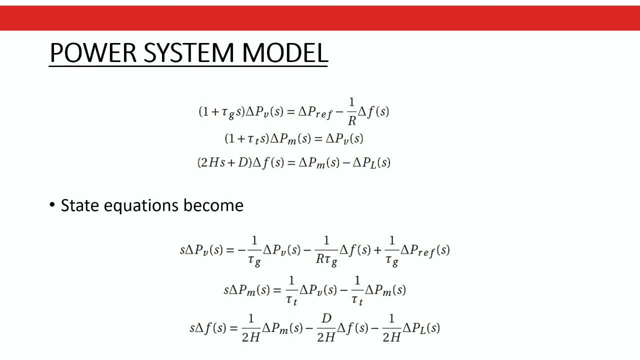 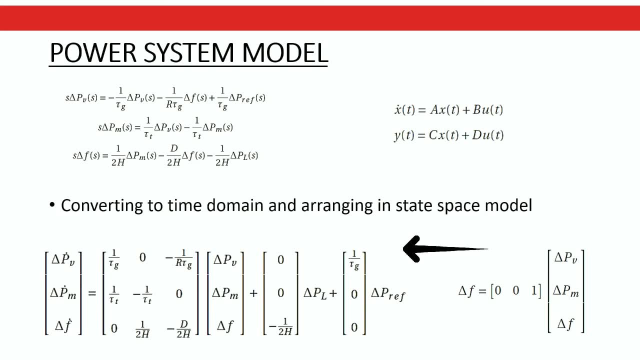 into s becomes a derivative in the t domain. so we get the final matrix form as this one. this is a two, two input, single output, as we see, delta pl and delta p ref. there is two input. for convenience, later on we will neglect this p reference. and this is the output equation. and so we are now next.